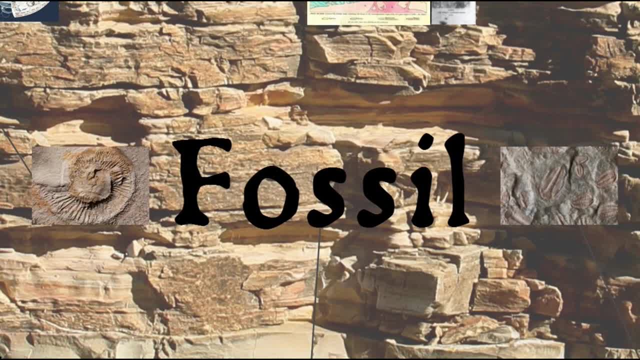 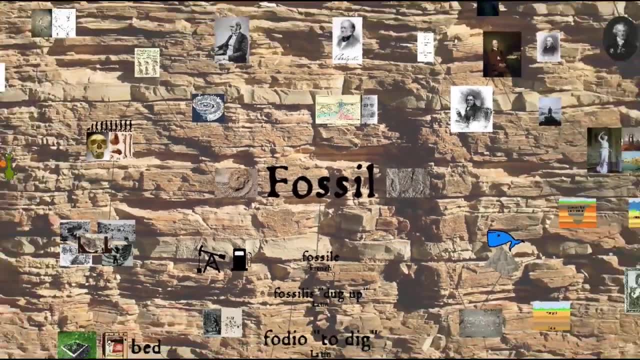 or, a little earlier, for the adjective form that fossil gained its more restricted but now most common sense of the petrified remains of ancient living organisms. And these two different but related senses tell us something about the scientific investigations of the 18th and 19th. 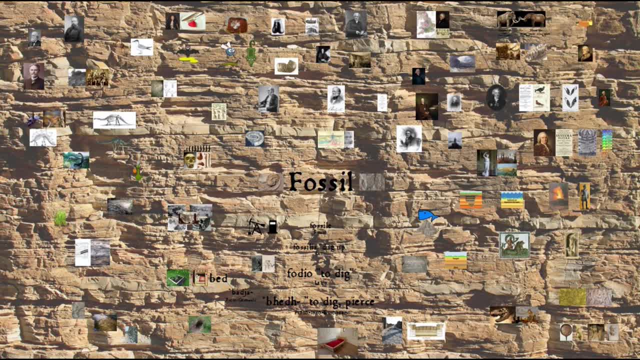 centuries, But more on that in a minute. Though the scientific study of fossils didn't really kick off until the 18th and 19th centuries, the scientific study of fossils didn't really kick off until the 18th and 19th centuries, though the scientific study of fossils didn't really kick off. 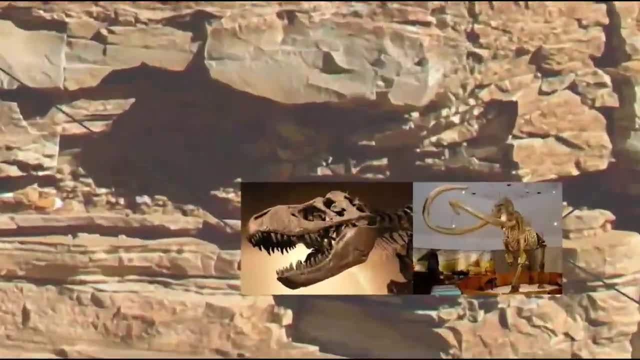 until the 18th and 19th centuries. though the scientific study of fossils didn't really kick off until the 18th century, people may have noticed them much earlier. Some scholars have argued that fossil remains of prehistoric megafauna may have inspired Greek myths about large monsters and 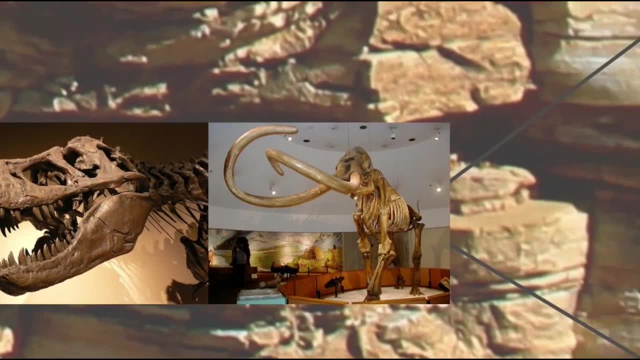 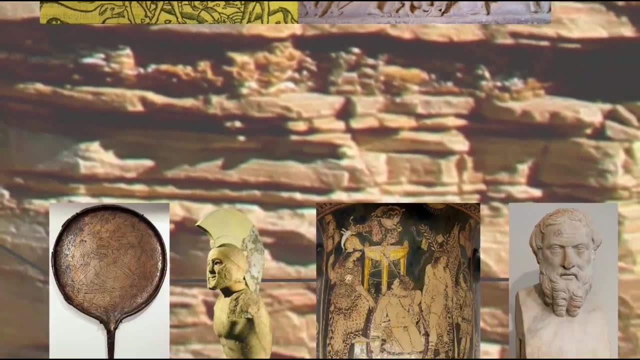 heroes of giant stature. For instance, finding mammoth tusks in an area that hadn't even heard about elephants yet may have led to stories of the gigantic Caledonian boar, And the Greek historian Herodotus reports that the Delphic oracle told the Spartans to find the bones of the hero Orestes. 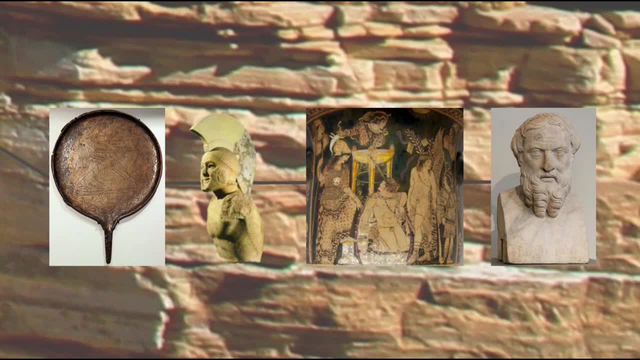 and when they dug up some huge bones near their border, they figured they'd found him and re-buried the skeleton. And so they dug up some huge bones near their border, they figured they'd found him. and when they dug up some huge bones near their border, they figured they'd found him and re-buried. 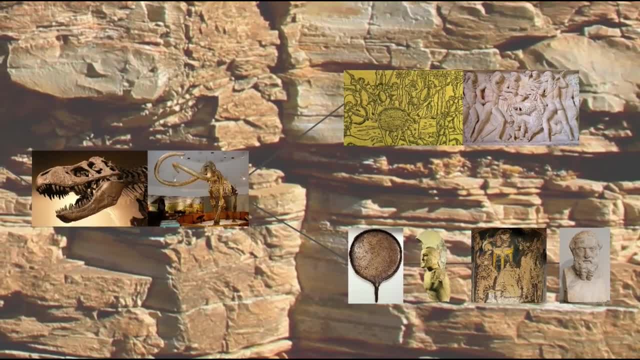 in a lavish tomb. According to one scholar, the Spartans' success with Orestes kicked off a pan-Hellenic bone rush, with every city wanting its very own monster bones. much like the bone rush of the 19th century, But more on that later too. There are many classical intrusions into this. 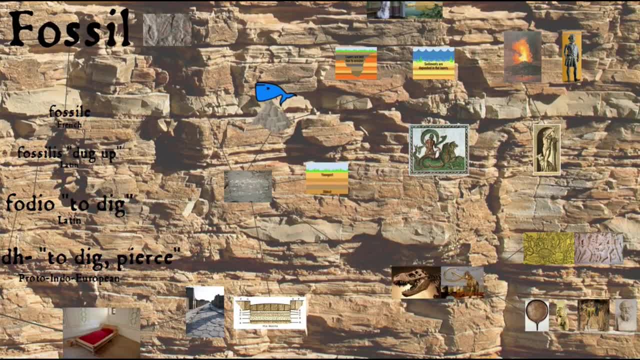 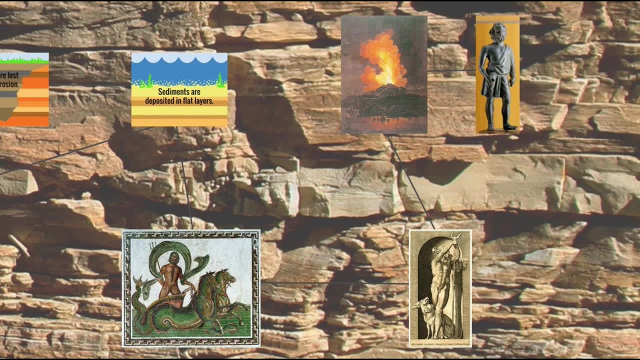 story, for instance, in the history of the complicated overlap between geology and paleontology. One of the major debates in 18th and 19th century geology was between the Neptunists and Plutonists. You see, people noticed that rocks were arranged in layers which came to. 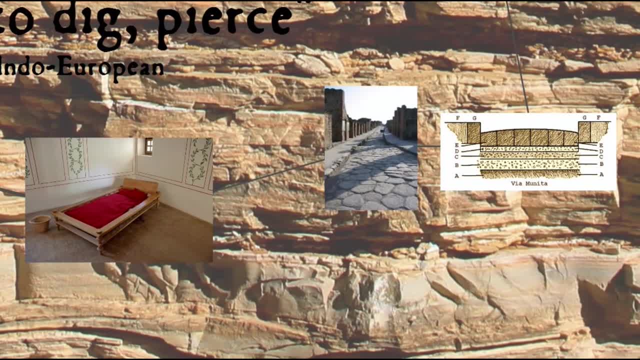 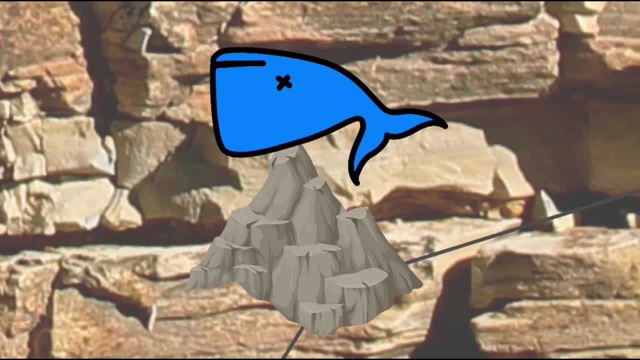 be known as strata, from the Latin for bed coverings or paved road, and also that fossils were contained in these strata And, most confusingly, there were fossils of sea creatures on mountaintops. So two schools of thought arose to explain this: Neptunists, named after the Roman. 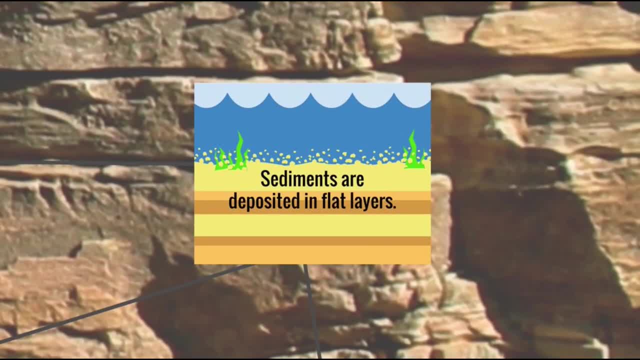 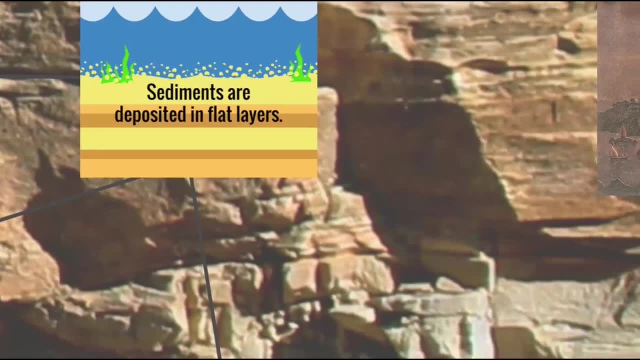 god of the sea said that the world was originally covered by a muddy ocean and rocks were formed as the water receded or dried up, leaving layers of sediment, and since then the earth had been basically unchanging. Plutonists, named after the Roman god of the underworld, pointed out that 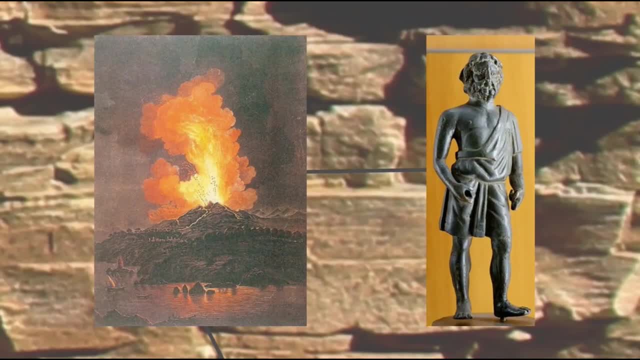 fossils weren't found in all strata and that they were only found on the surface of the ocean, And maintained that new rocks were formed by a continuing process of volcanoes named after the Roman blacksmith, god, Vulcan and earthquakes, though this left open the question of fossilized 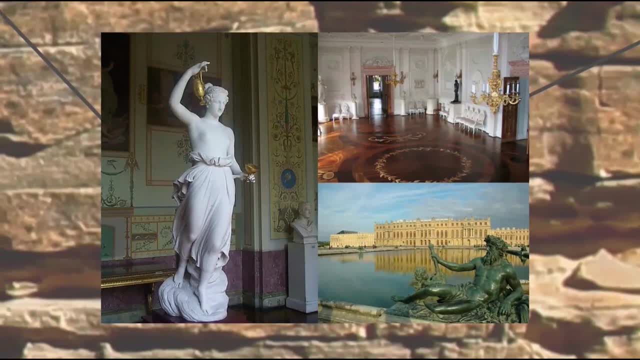 shells on mountaintops. Meanwhile, the 18th century was also the age of reason and enlightenment. Classical harmony and symmetry were the aesthetics of the day, and this way of thinking governed the sciences as well. The great taxonomist Carl Linnaeus set about classifying all living things. 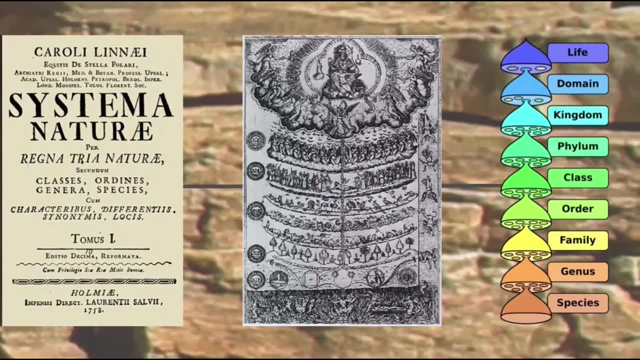 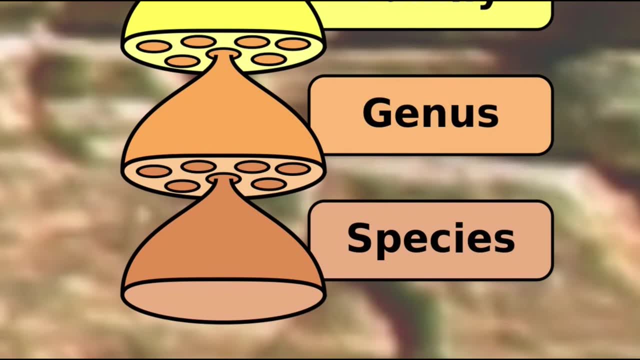 with the belief that God had created a perfect and unchanging order and all humans had to do was identify them, He developed the binomial naming system that we still use today, made up of two Latin names to identify the genus- Latin for clan or family- and species- Latin for type or appearance. 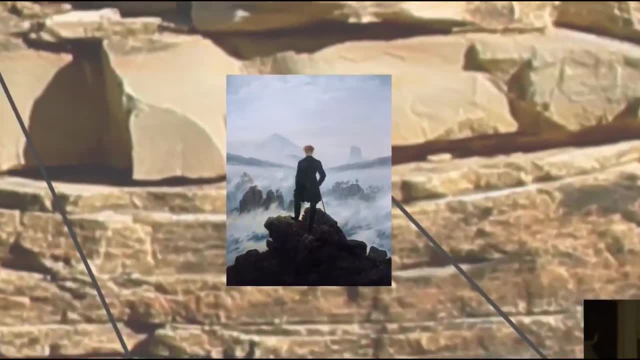 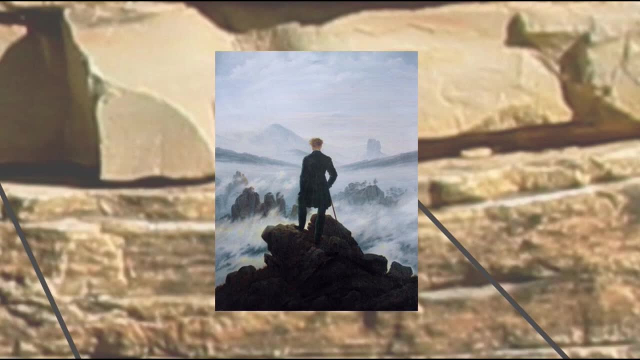 But toward the end of that century and into the next, as the unruly passions of Romanticism, which was really into the chaos of nature, began to challenge the neoclassical order, the ordered view of the natural world was about to shatter as well. Continuing in Linnaeus' task, 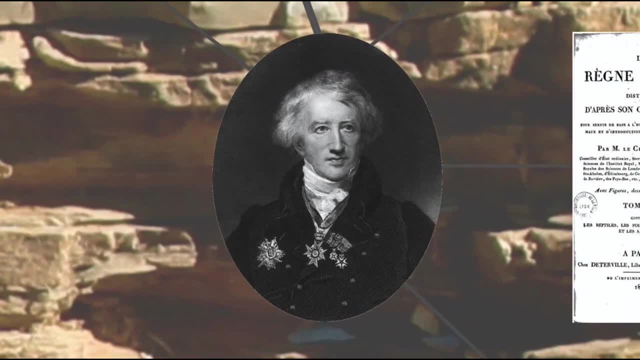 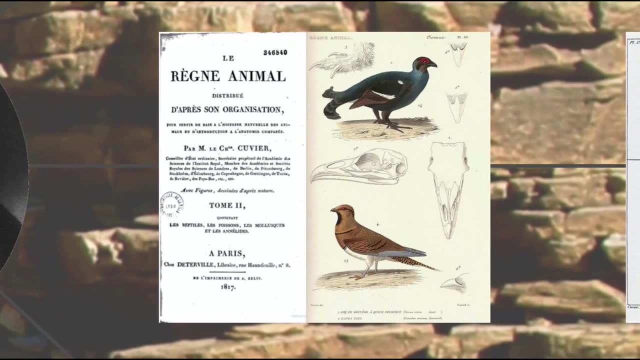 of classifying animals was Georges Cuvier, who practically wrote the book on comparative anatomy- could reconstruct the shape of an entire animal from a single bone through the principle of the correlation of parts. The sharp tooth of a carnivore implied a particular jaw shape. 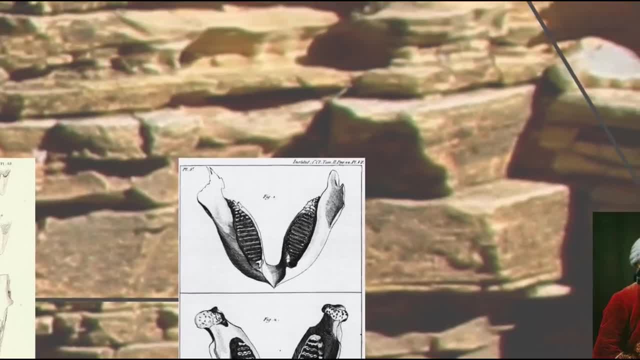 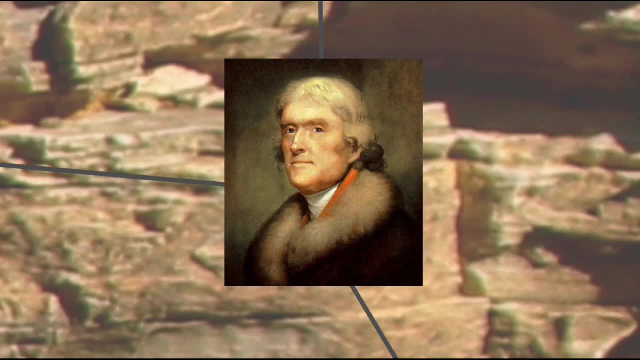 which implied a particular skull shape and so forth. This was demonstrated when American President Thomas Jefferson, a fossil fanatic, started a campaign of sending over to Europe specimens of animals of unusual size to counter the French naturalist, the Comte de Buffon. 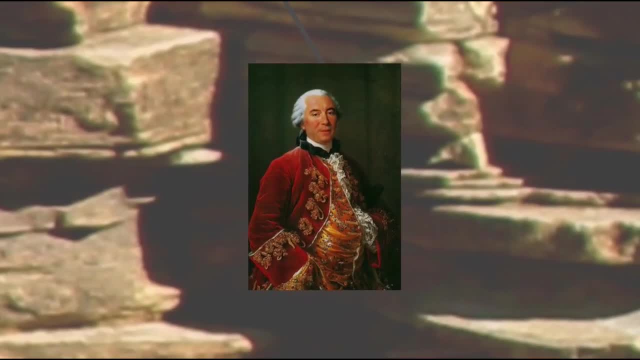 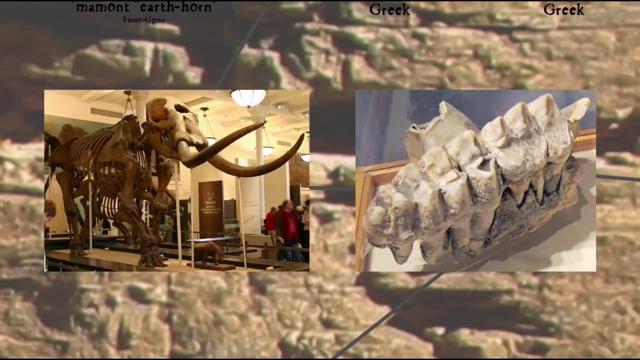 who claimed American animals were small and degenerate compared to the European ones, and in doing so inadvertently kicked off American paleontology. Cuvier, starting with a single tooth that the Americans had sent, was the first to formally describe and name the American mastodon. and I bet you didn't expect that word to mean nipple tooth, from the Greek for breast and tooth. because of the titillating shape of the teeth, They were initially confused with mammoths until Cuvier's work established them as a distinct but related species- The name mammoth, by the way. 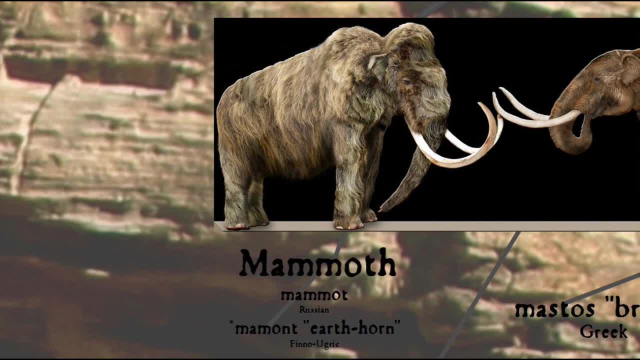 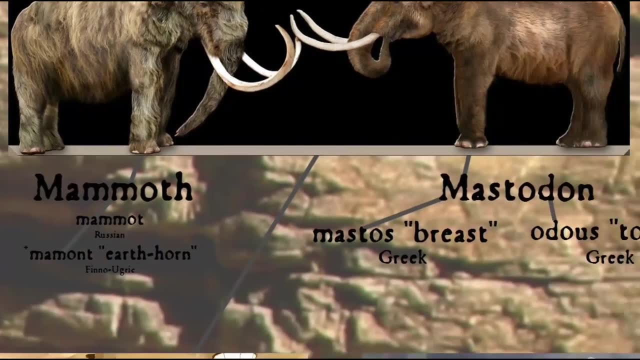 comes through Russian, ultimately from the Finno-Ugric root meaning earth horn, because mammoth remains having been found in the ground, they were believed to have been a burrowing hole and, as a side note about Thomas Jefferson, the word mammoth was first used as an adjective. 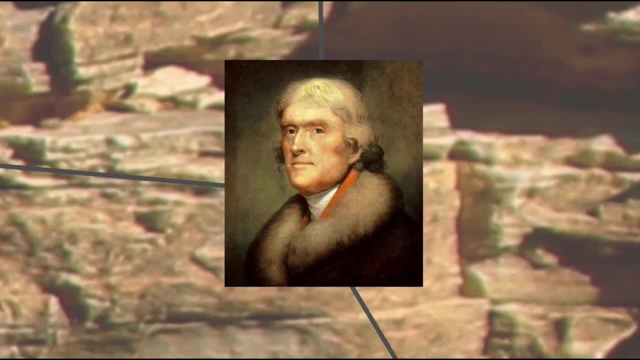 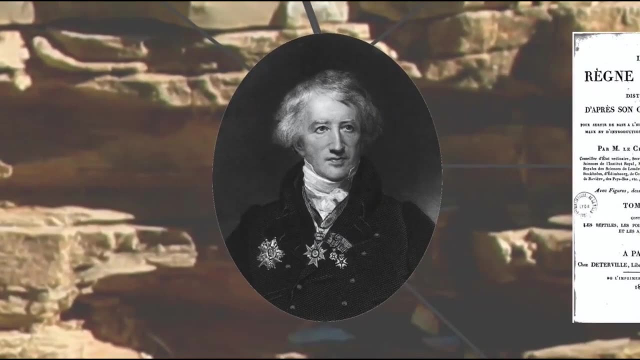 meaning huge, to describe not an animal of unusual size but a cheese wheel of unusual size that was presented to the President. But getting back to Cuvier, he also studied the strata and noticed that certain fossils were only found in certain layers and then disappeared, and this led him to 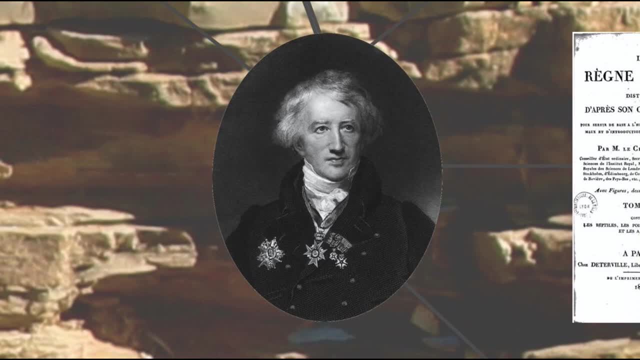 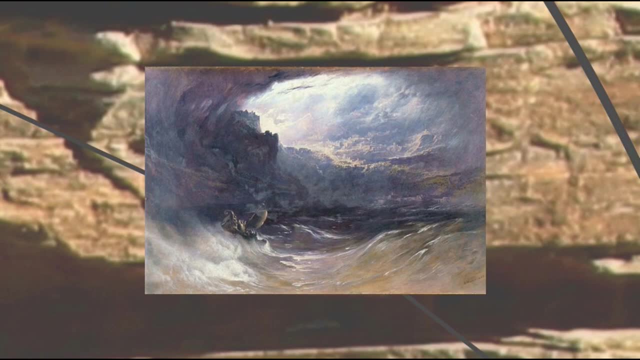 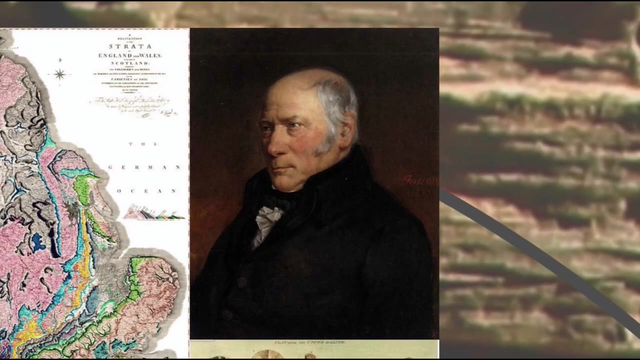 be one of the first to really suggest the idea of extinction. He proposed the idea of catastrophism, which fit in with the Neptunism of the geologists. Cuvier's findings in France fit with those of an Englishman, William Smith, who is so important to. 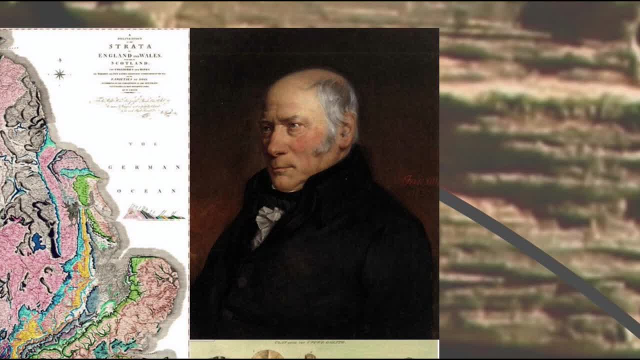 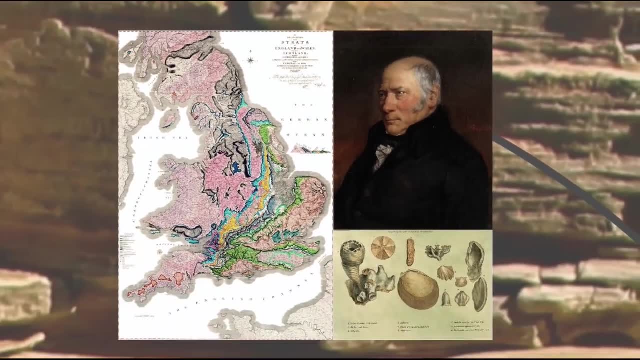 the study of strata that he is sometimes credited with coining. the term stratigraphy- the first recorded instance of the word- refers to his work and was nicknamed William Strata Smith. Smith was a surveyor working for a coal company and realized he could work out the relative ages. 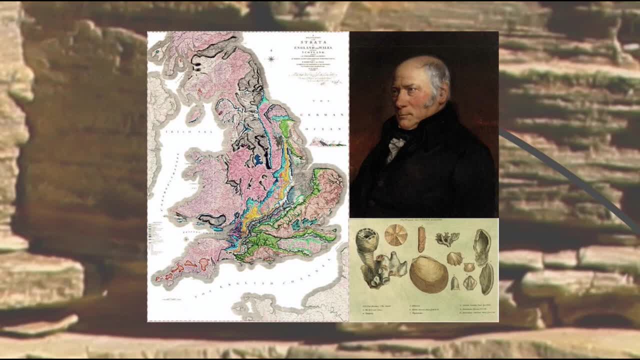 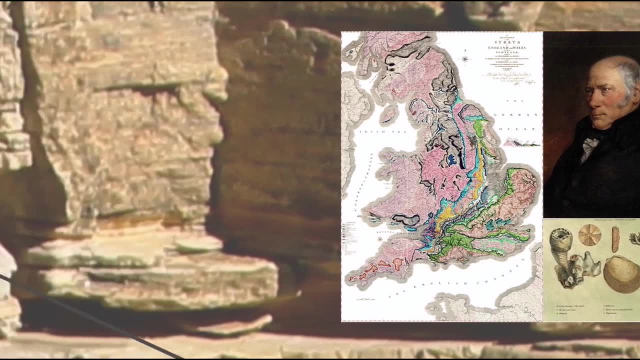 of strata by the type of fossils they contained and, after much study, produced a geological map of Britain showing all the different strata, a map which was sadly, immediately plagiarized. Another proponent of the flood theory was an eccentric theologian-cum-geologist and 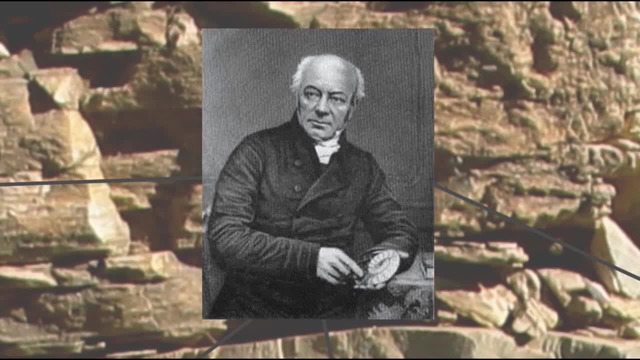 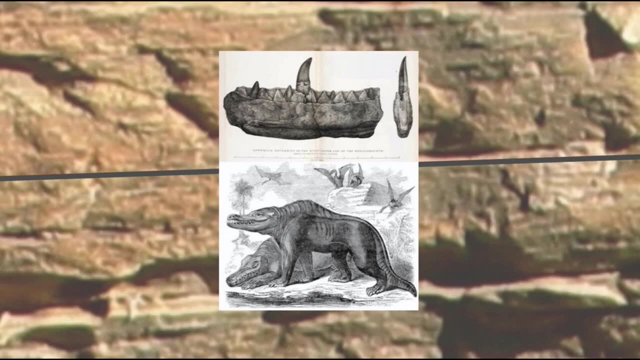 paleontologist William Buckland, who was also significant as the first to formally describe a dinosaur, which he called Megalosaurus, from its fossil remains. The name Megalosaurus is from Greek, meaning big lizard, and perhaps unfortunately replaced the Latin name originally given to the. 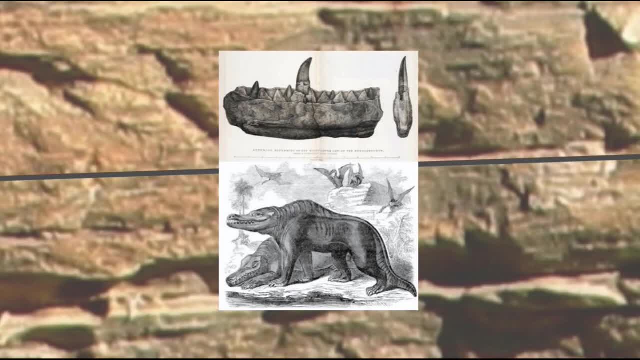 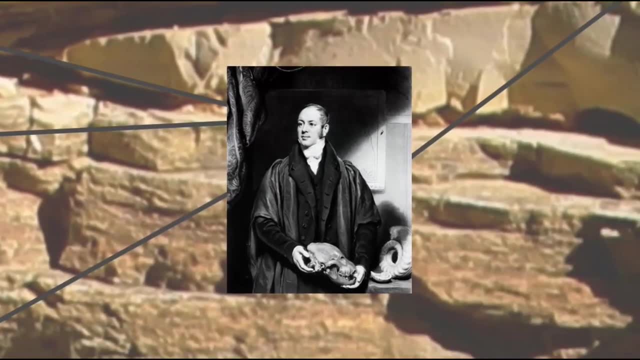 fossilized end of a femur, which was the first of its bones to be found scrotum humanum because of its ripped out meat. Well, As for the eccentric Buckland himself, he preferred to do his fieldwork while wearing his academic 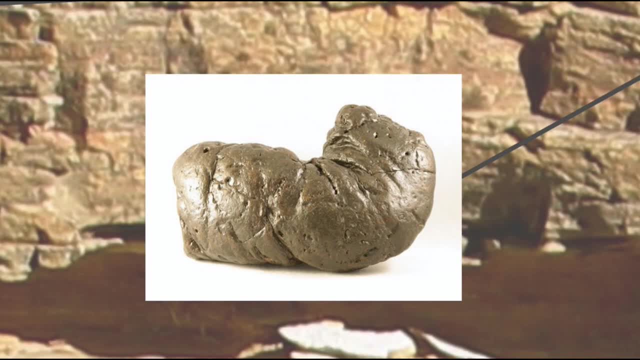 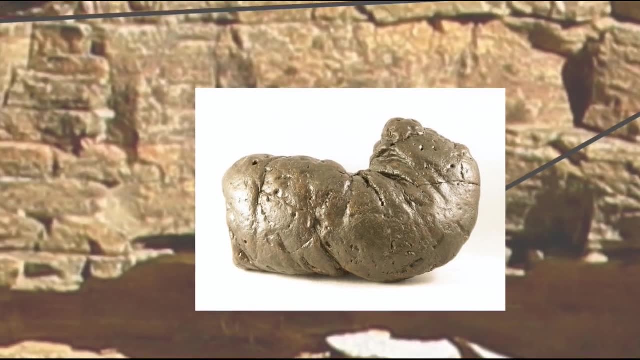 robes. and, having pioneered the study of coprolites, fossilized faeces, he had a table made with inlaid specimens and only told his guests what it was made out of after they'd eaten off it. He also had odd tastes in food, being obsessed with trying many unusual animals. 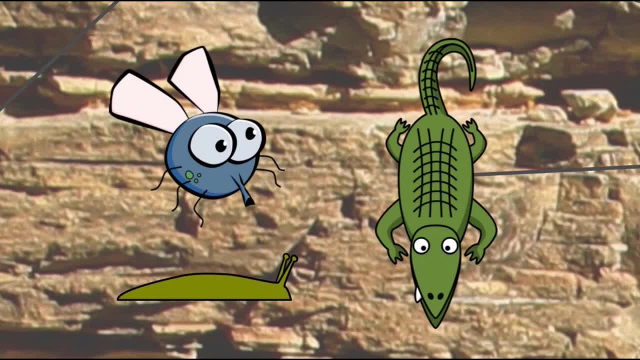 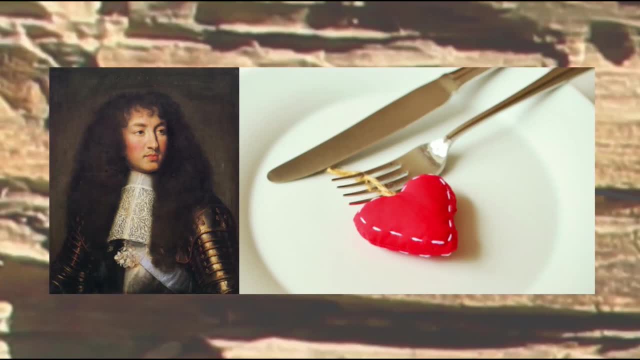 such as sea slugs, crocodile and blue bottle flies and was apparently fond of toasted mice. He was also rumoured to have eaten the mummified heart of Louis XIV, and he was purported to have properly identified a dark stain on the floor of a cathedral which was thought to 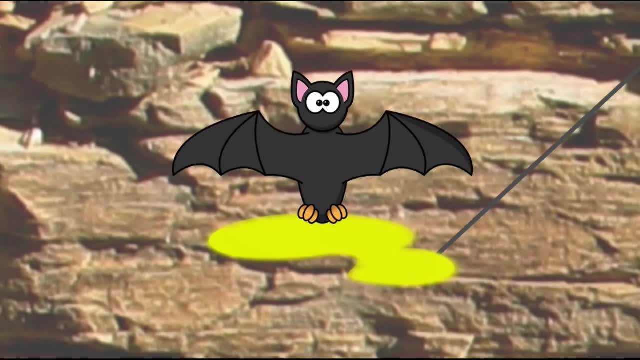 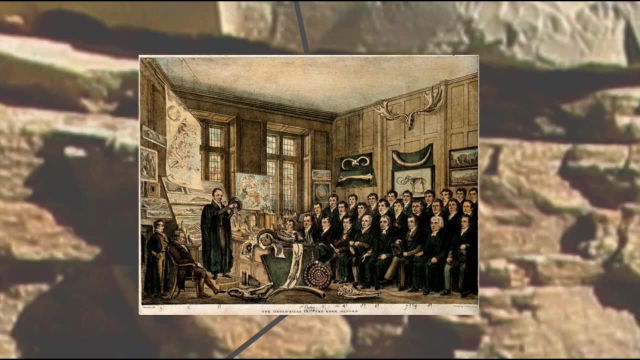 be the blood of a martyr, as actually bat urine by tasting it. But all of this eccentricity didn't go to waste, as he was known for using humour and buffoonery in his lectures at Oxford University to keep his students interested and entertained. 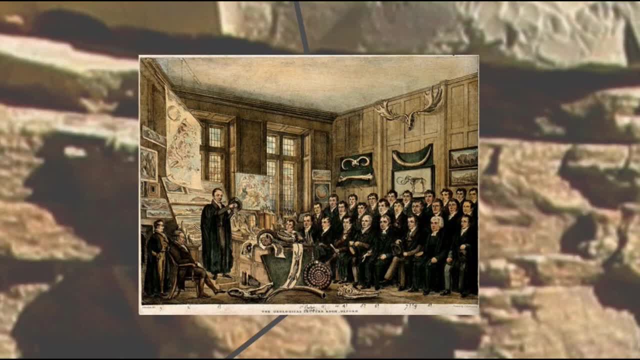 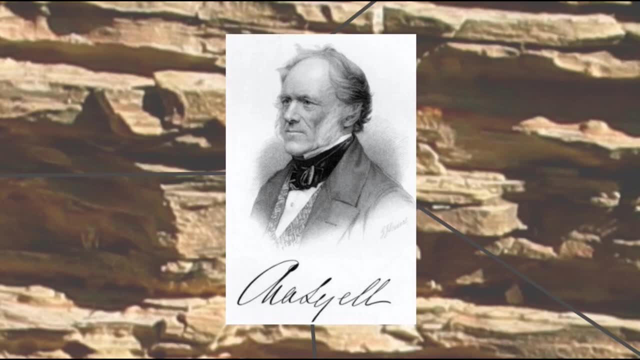 Shocking, And Buckland is particularly important to this story because of one of those students, Charles Lyell. Lyell, disagreeing with his wacky teacher Buckland and the other Neptunist synctastrophists, instead turned to the work of a man who died the year Lyell was born. 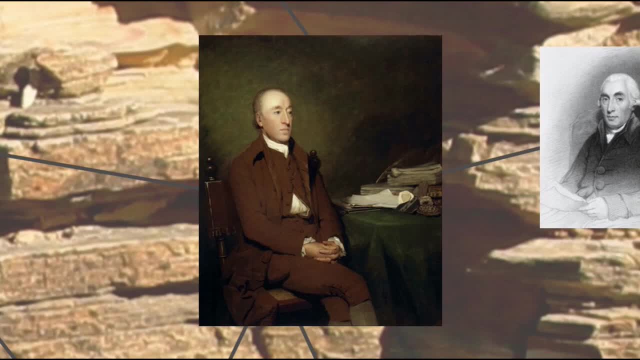 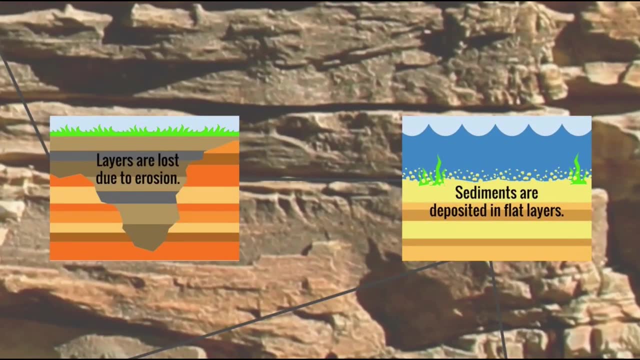 This farmer-turned-geologist, the Scotsman James Hutton, who held to the Plutonist school, proposed the theory of uniformitarianism—that the gradual and ongoing processes of erosion and sedimentation, along with ongoing volcanism, could account for the geological evidence. 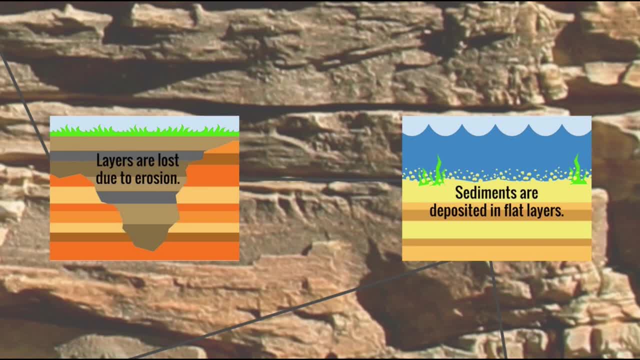 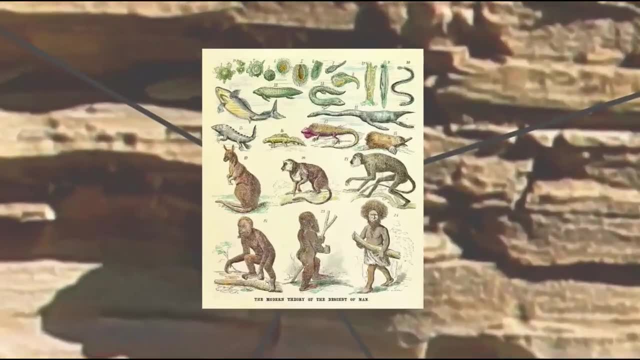 and that these processes must have been happening in the same way for a very long time, with no need for great catastrophes or earthquakes. He even applied this gradualistic notion to living things, with a kind of proto-theory of evolution through natural selection. 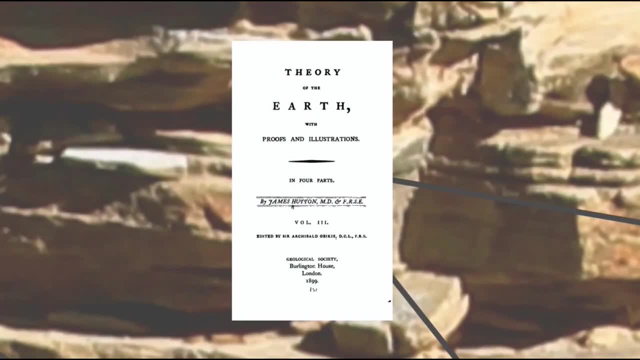 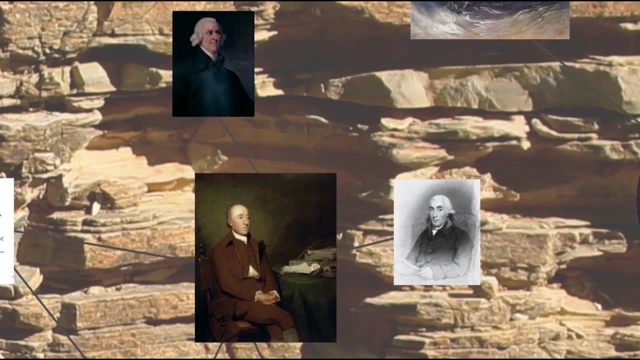 But unfortunately Hutton was such a bad writer that his ideas came close to going completely unnoticed. Hutton was part of the so-called Scottish Enlightenment and as such palled around with other Scottish notables of the day and along with moral philosopher Adam Smith and 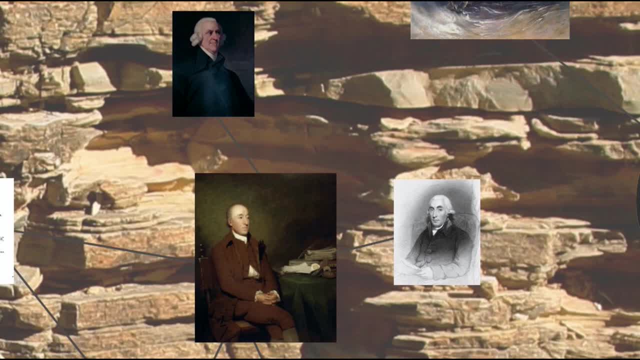 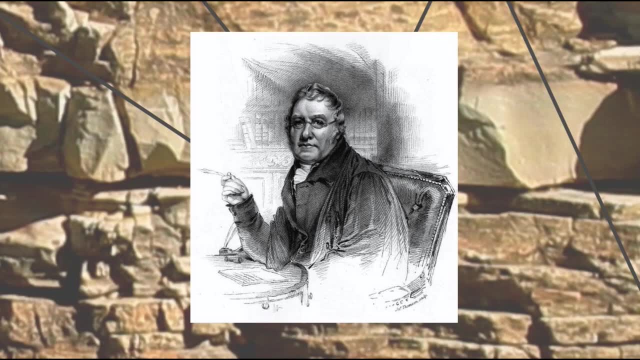 chemist Joseph Black, formed a dining club called the Oyster Club, soon to be joined by mathematician John Playfair. Playfair, realizing Hutton's writings needed to be written in a way that would make sense, needed to be reworked, wrote a summary of them explaining Hutton's uniformitarianism. 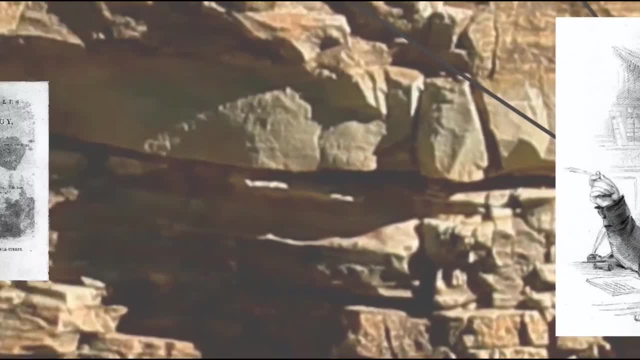 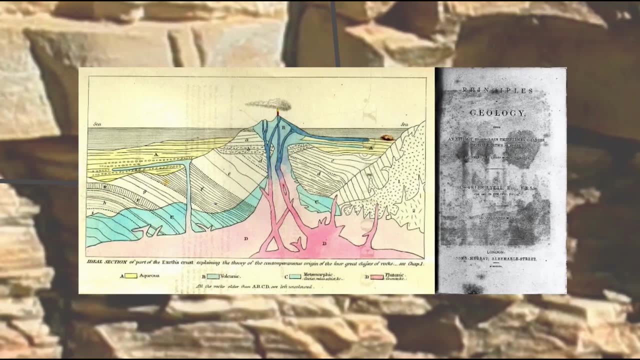 And it's through this that Lyell got on to the idea. Lyell wrote his own book promoting and popularizing the idea, also providing the additional evidence of fossils in strata that ran under volcanic mountains, which demonstrated the extreme age and slow pace of everything. 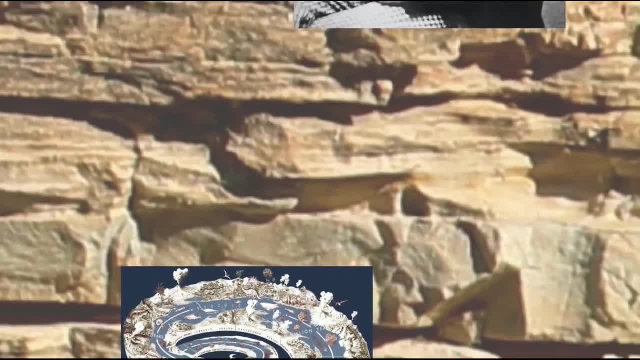 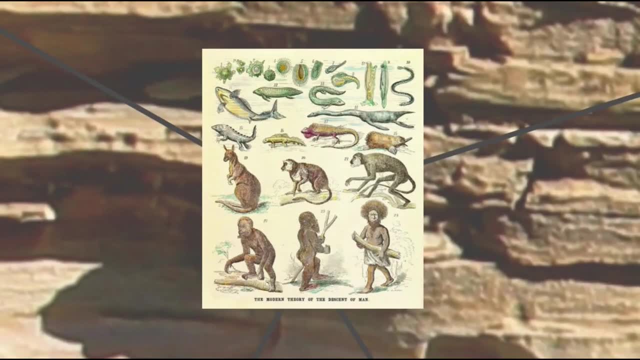 And this book made a big impact on Lyell's friend Charles Darwin, who went on to formulate his own idea of evolution through natural selection, seemingly unaware of Hutton's earlier musings. So Darwin's theory of evolution is the same as Hutton's earlier musings. 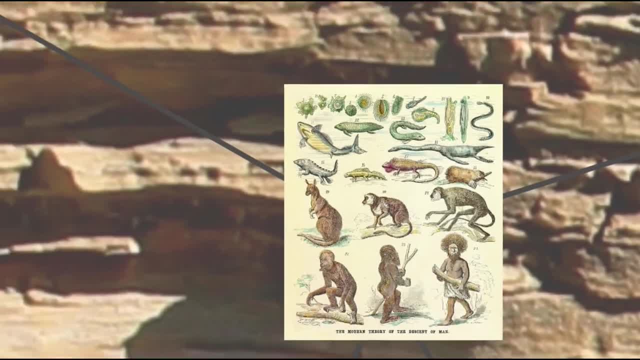 So Darwin's theory of evolution is the same as Hutton's earlier musings. So Darwin's theory of evolution is the same as Hutton's earlier musings. Darwin's theory only further inflamed the bone rush going on among the fossil hunters for further proof of evolution and extinction and the search for the so-called missing links. 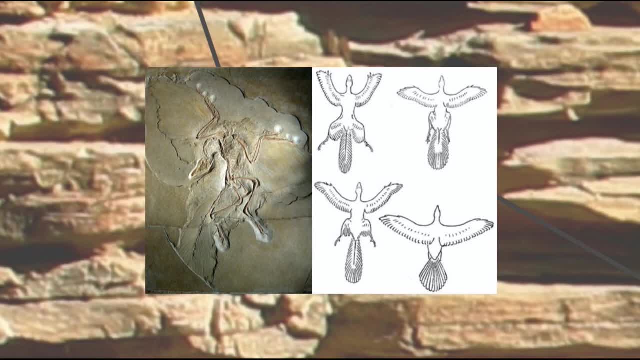 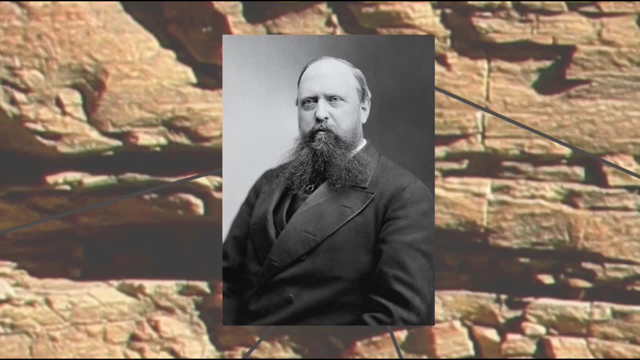 between one species and another, such as proof of the theory that birds were descended from dinosaurs. American bone hunter Othniel Charles Marsh supported that theory with his study of the first fossil specimens of a toothed bird, Ichthyornis, from the Greek meaning fish-bird. 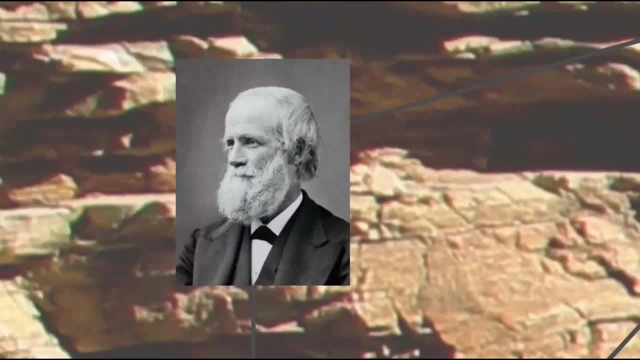 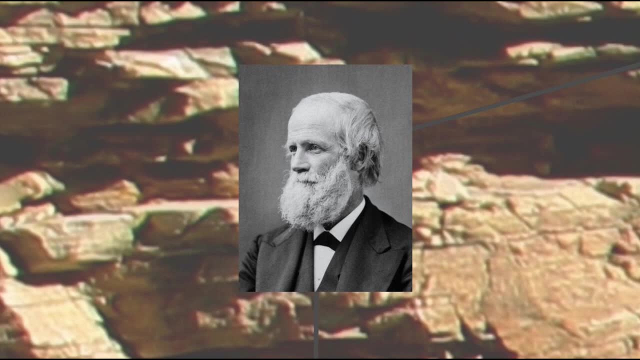 Marsh himself hadn't uncovered the fossil, which was actually found by geologist Benjamin Franklin Mudge. Mudge had originally had an arrangement to send fossil finds to Edward Drinker Cope, Marsh's hated rival in what has become known as the Bone Wars. but Marsh convinced Mudge. 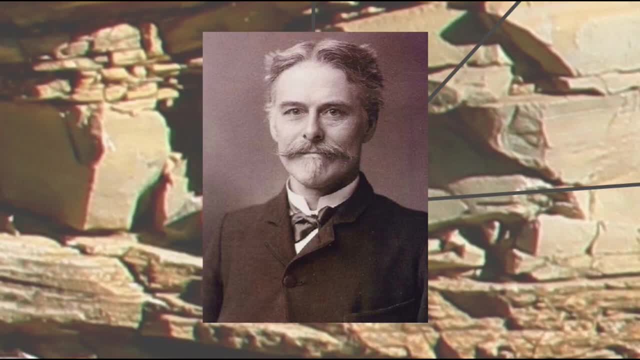 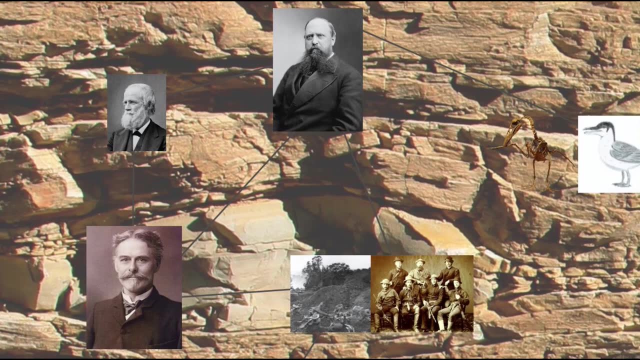 to send the Ichthyornis fossil his way, so Marsh beat Cope out as the classifier of this crucial fossil. The Bone Wars was the intense and often underhanded professional and personal competition between Marsh and Cope, two of the most important paleontologists of the 19th century. 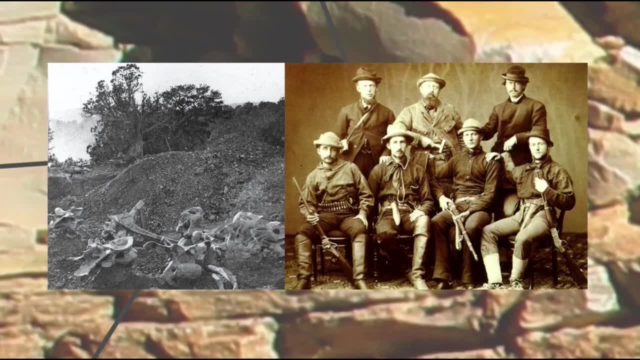 Not only did they attack each other in print, but they also attacked each other in the scientific world. They poached each other's quarries, descending to bribery, theft and even dynamiting fossils to keep them from falling into each other's hands. 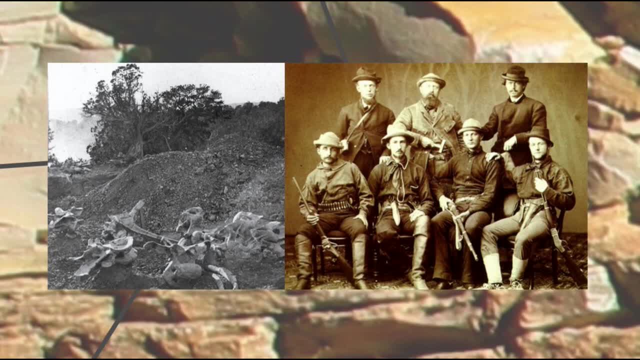 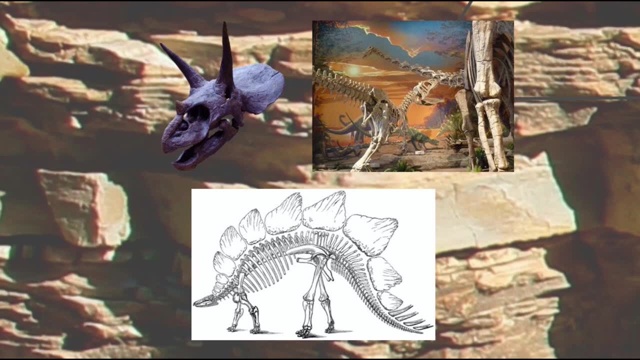 And, at the end of it all, both were left broken and financially ruined. men, Though often destructive, their competition to discover the most species led to the classification of some of the most iconic dinosaurs: Triceratops, Allosaurus, Diplodocus and Stegosaurus. 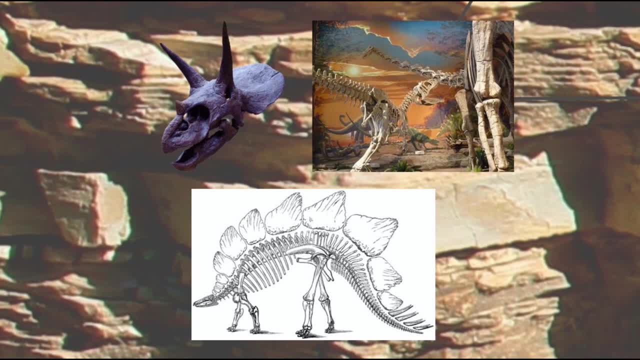 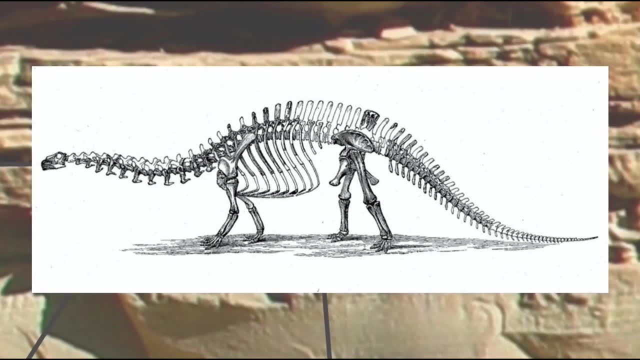 Sometimes their haste to one-up each other led to mistakes like misidentifying as new animals fossils of species that had already been discovered, As in the famous case of Brontosaurus. Marsh had discovered and named the Brontosaurus from the Greek meaning thunder, lizard, but 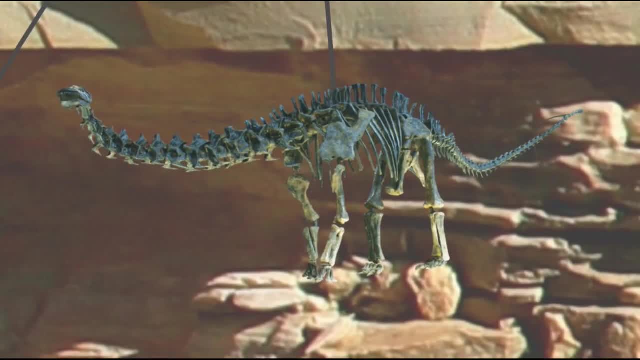 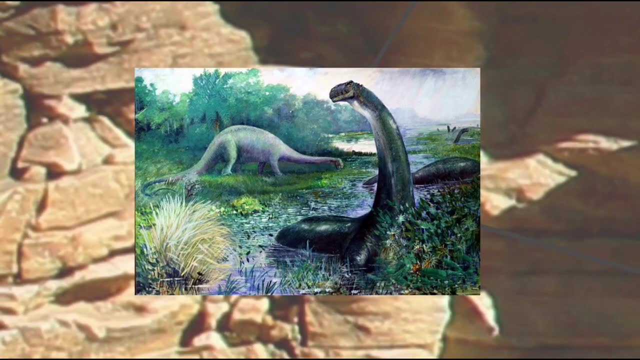 it was later decided that the fossil find was really a specimen of the previously discovered Apatosaurus, so officially, the name Brontosaurus was dropped, except in the popular imagination, where it persisted as one of the most famous dinosaur species. But recently, in early 2015,, a reexamination of the fossil has shown that there were actually. 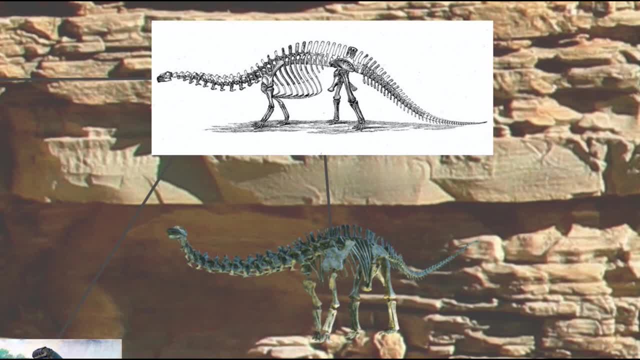 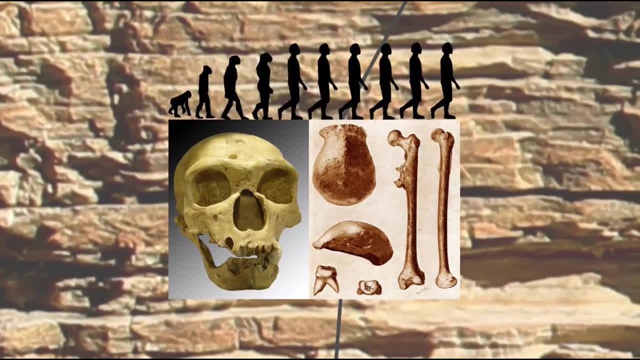 I'm sure Marsh would have been just as pleased as the eight-year-old dinosaur lover in all of us. I'm sure Marsh would have been just as pleased as the eight-year-old dinosaur lover in all of us. Of course, fossil evidence for the evolution of humans from earlier primates was also sought. 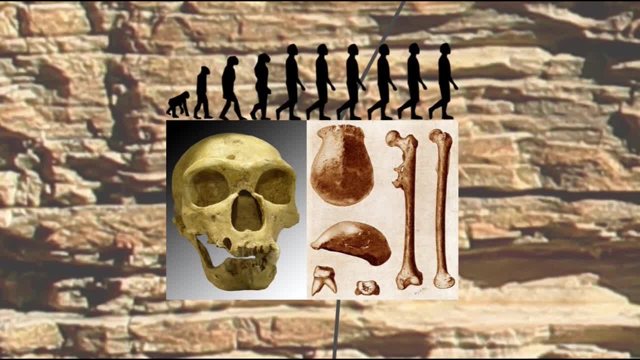 and found too, including such species as Javaman, now classified as Homo erectus, from Latin meaning upright person, and Neanderthal so called because it was first discovered in the Neander Valley near Dusseldorf and the principles of stratigraphy became a central. 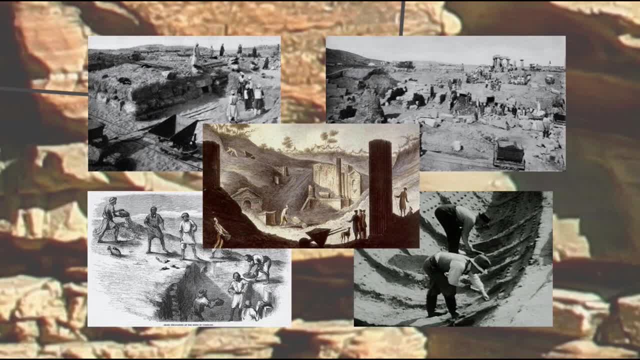 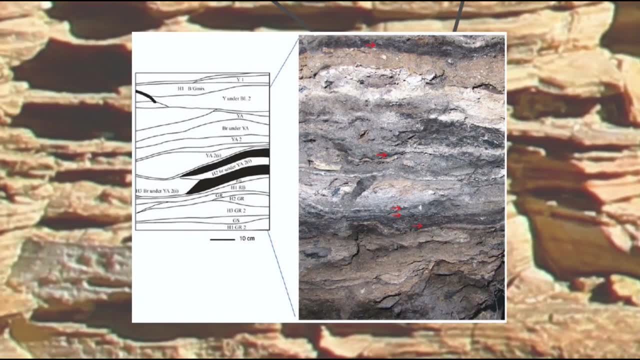 precept of the study of the physical remains of human activity, such as artifacts or structures, In other words archaeology. One interesting recent archaeological discovery is the Archaeological Survey, which is a study of the oldest known remains of a bed made by early humans in the Subudu cave in 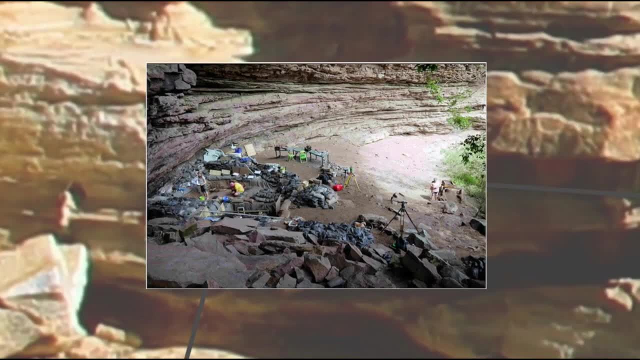 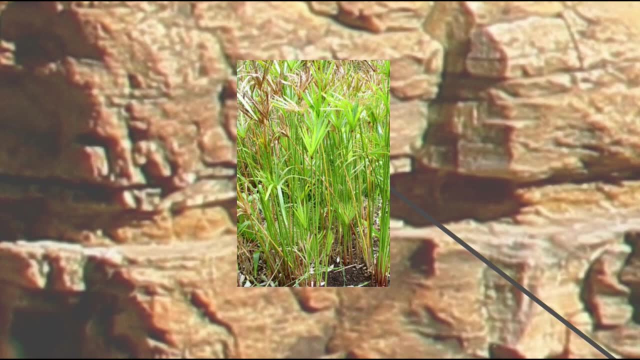 what is now South Africa. some 77,000 years ago, This mattress was made out of layers of sedges which have insecticidal properties to keep the pests away, with a layer of leaves on top, and was big enough for a whole family. 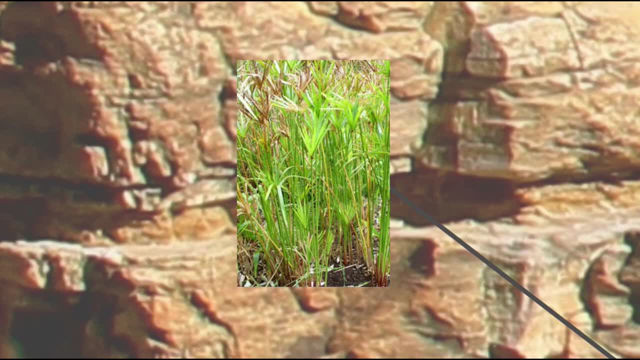 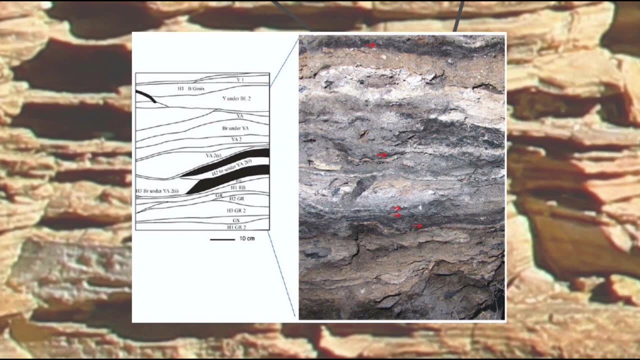 to sleep, on giving us clues to the social arrangements and behaviours of early humans. What's more, it appears to have been used over a period of 39,000 years, being periodically burned and then re-layered with fresh sedges and leaves, so the bed itself is made up of. 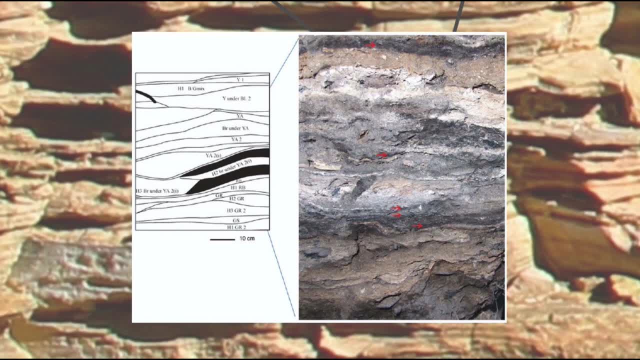 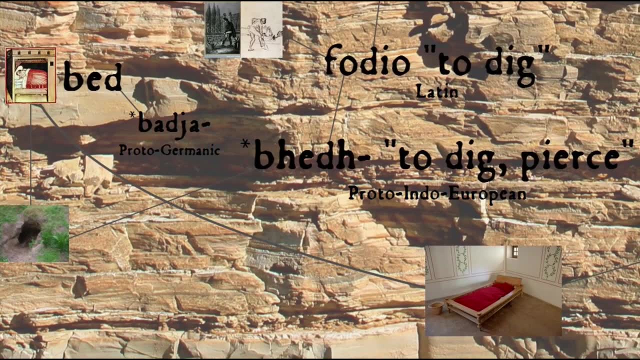 strata or bed coverings in Latin, remember, of fossilized plants accumulated over thousands of years, Which is particularly appropriate since the word bed comes from the same Proto-Indo-European root. that gives us fossil only through the Germanic branch of languages instead of Latin. It's a matter of some speculation why a word that meant to dig came to mean a place for sleeping, but perhaps it had to do with the notion of a hollow dug out of the ground like a den, giving us a linguistic clue to the sleeping arrangements of the past. 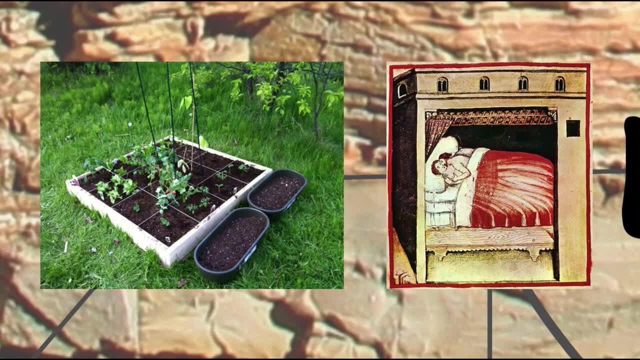 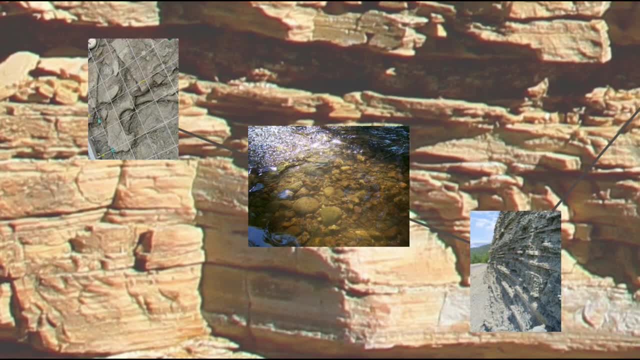 Perhaps the word bed could refer to a place to sleep as well as a garden bed where you might dig, And by the beginning of the 17th century, the word bed could refer to a layer or stratum, like a geological bed, a lake bed or a bone bed containing fossils. 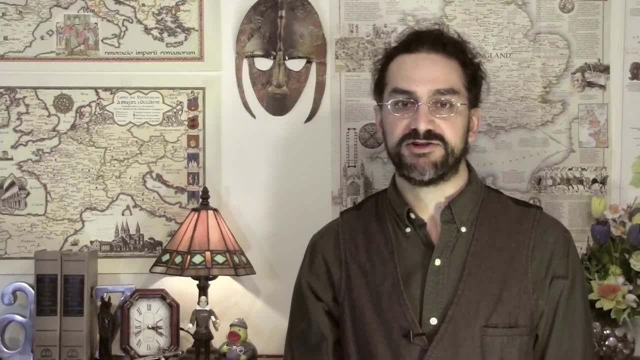 So this video is a bit like uncovering the strata of history and etymology, and like Cuvier puzzling out the shape of an entire organism starting from one small bone. we've puzzled out this whole story from one word's etymology. 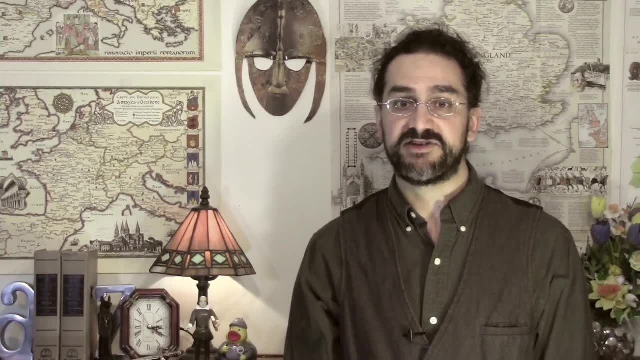 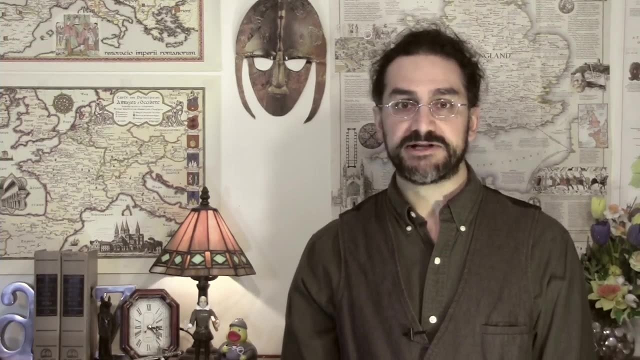 And, like the fossil mattress, the etymology of bed gives us a glimpse of the deep and distant past. Can you dig it? Thanks for watching. If you've enjoyed these etymological explorations and cultural connections, please subscribe to this channel to help me make more videos. 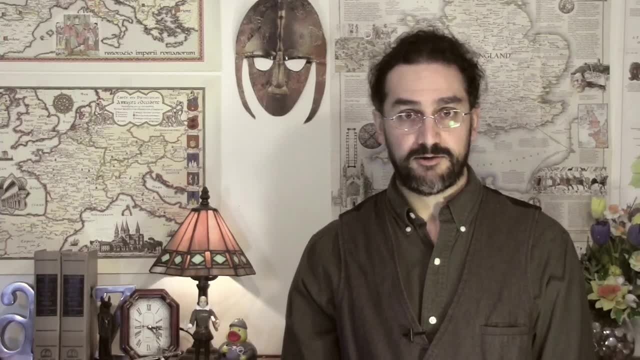 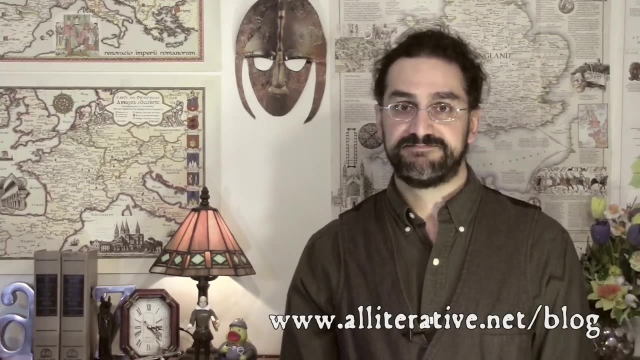 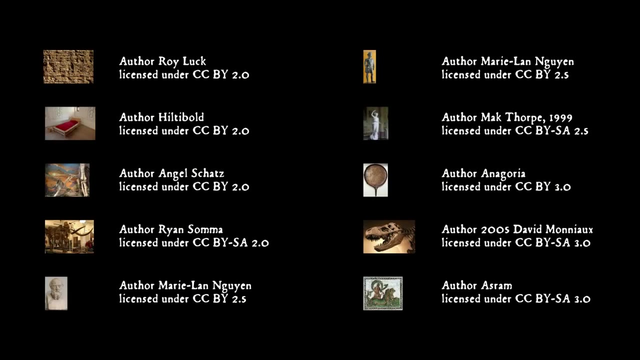 You can also sign up for email notifications of new videos in the description below. Leave a comment or question or tweet at alliterative. You can also read more of my thoughts at my blog at alliterativenet. I'll see you in the next video. Bye, Bye. 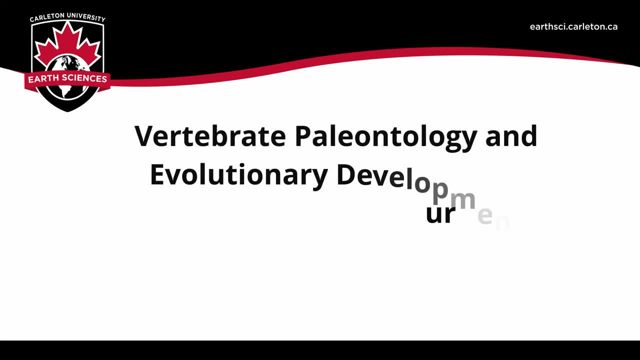 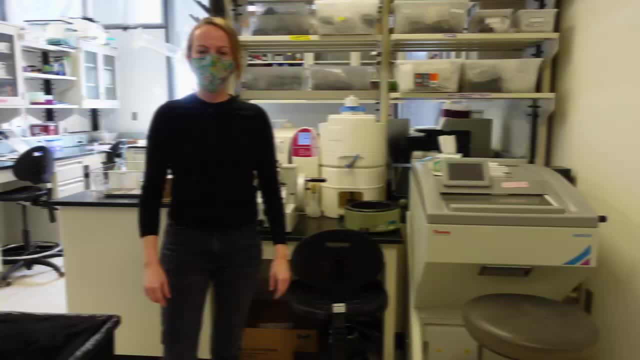 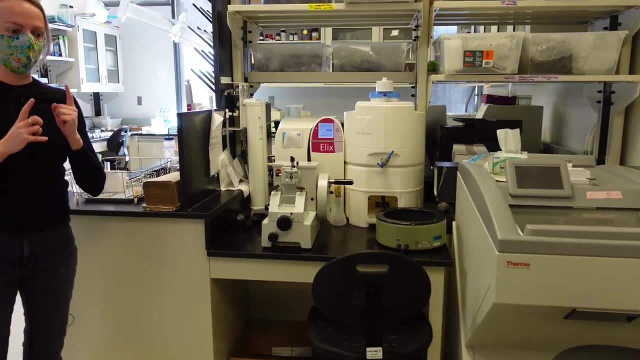 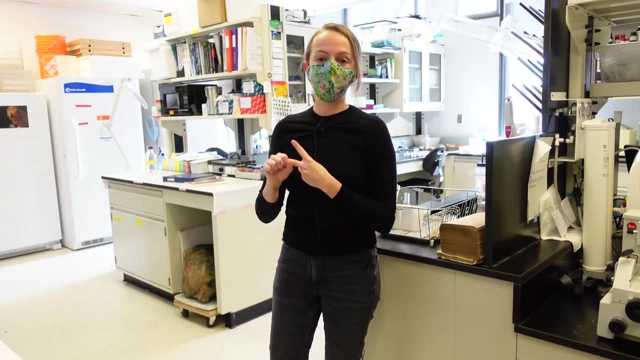 Hi, welcome to the Vertebrate Paleontology and Evolutionary Development Lab. So in this lab we do a couple of different things. For one, we look at the fossil record of our animals, and then we also look at the bones of some living animals to help us.